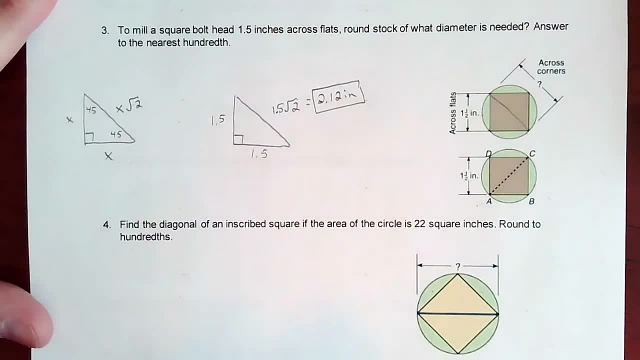 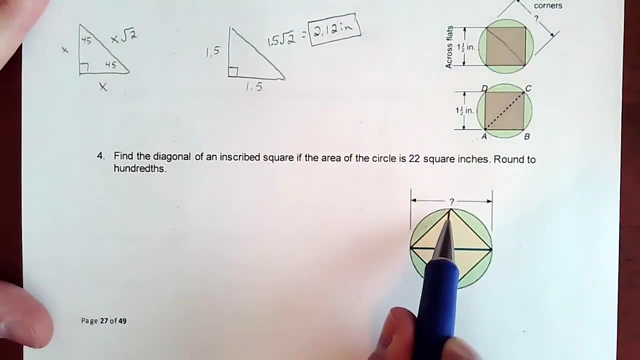 And so we have 2.12 inches across. So if we do one more, we're going to find the diagonal of an inscribed square. So an inscribed square- inscribed just means you're going to have this square that's drawn inside of the circle- 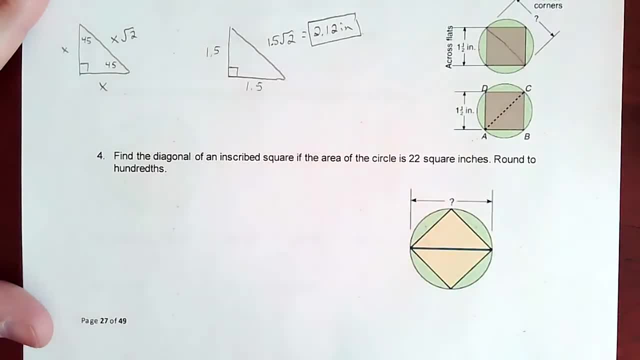 Notice the corners, because it's a square. the corner should all kind of touch at points on the circle. It says: find the diagonal. So the diagonal is also the diameter of the circle. So it's the diagonal of the square, but it's the diameter of the circle. 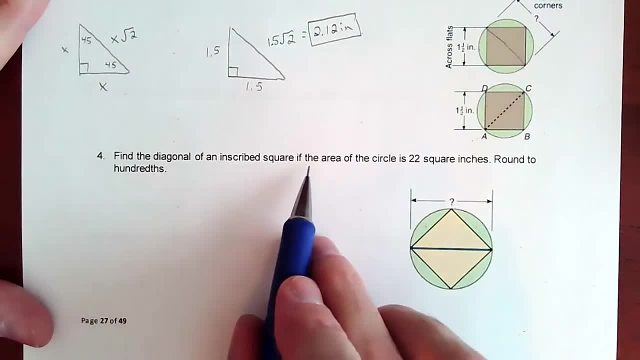 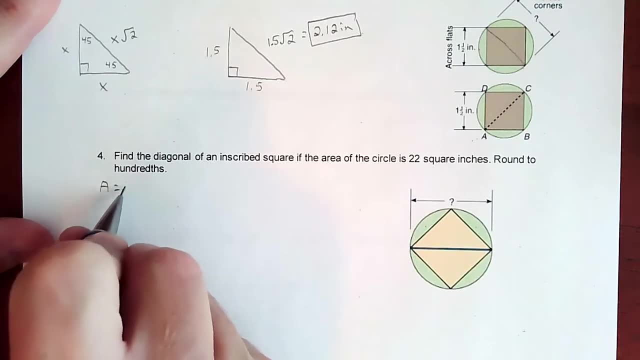 It's the same idea- The diagonal of the inscribed square if the area of the circle is 22 square inches. So the only thing that I can get out of area, which is actually very helpful, is: this is your formula for area. 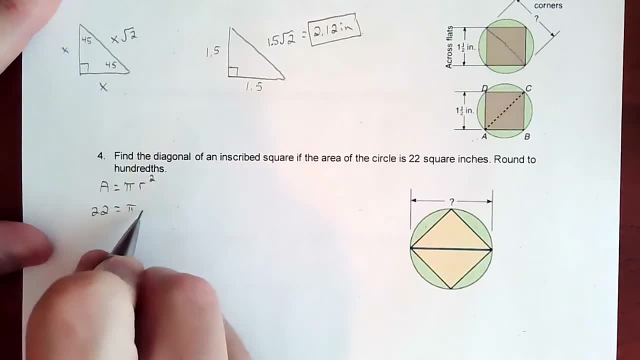 They tell us that it's 22. And what I can find out of that is: I can find the radius. The radius would be from the center to the edge, which is going to be half of our diameter, which is half of our diagonal. 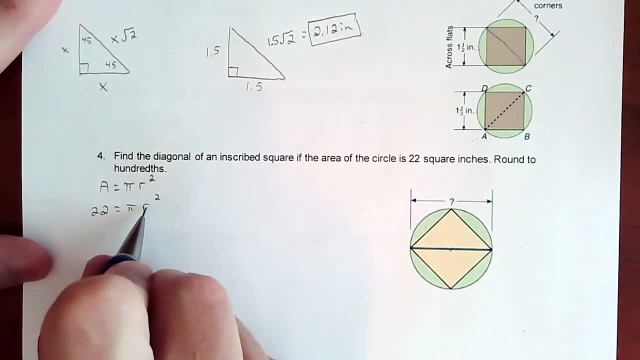 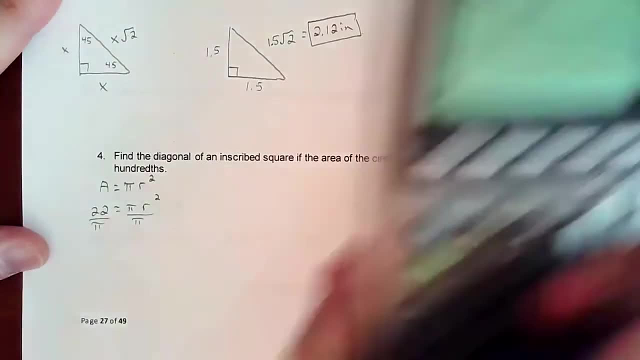 So the radius would be pretty helpful actually. So let's solve for that. So to get r squared by itself, we're going to divide by pi, Right? So I'm going to let the calculator kind of store a bunch of stuff for me. 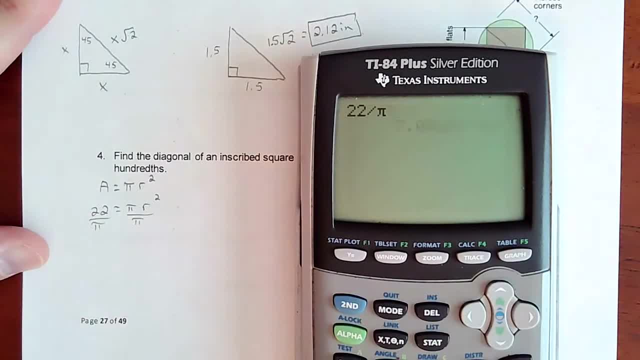 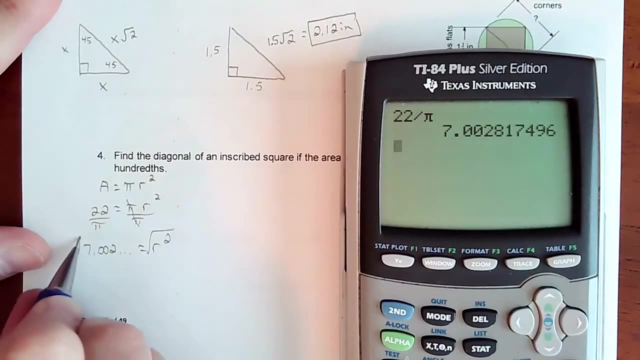 So we have 22 divided by pi, Right? So pi is some value, but I'm not going to round it. 7.002, blah, blah, blah equals r squared, because the pi's would cancel. Then we want to get rid of the square by square rooting. 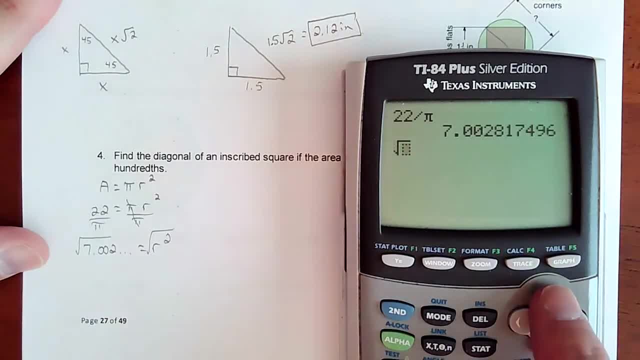 So if we square root the right, we're going to have to square root the left, So we're going to square root that value, All right, And I want to be as accurate as possible, So I squared the whole thing And the radius is 2.2.. 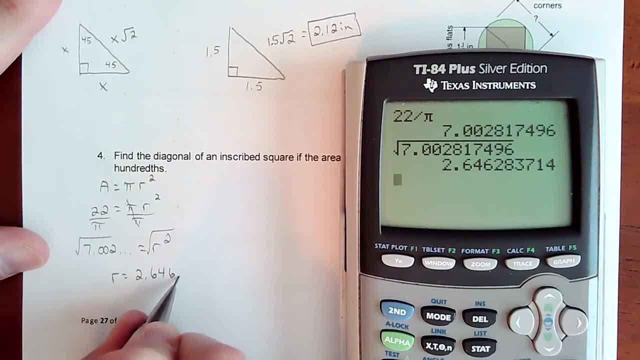 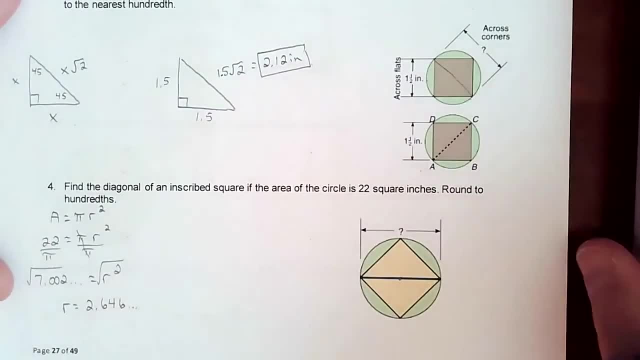 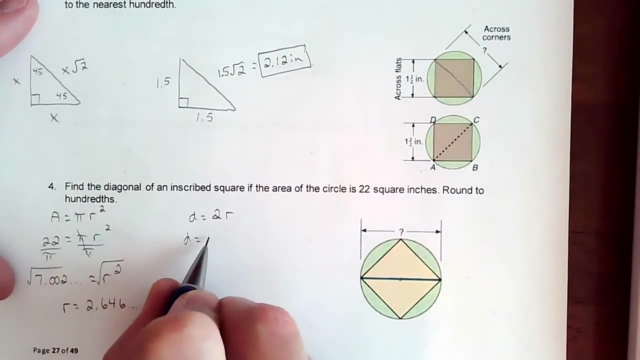 0.646, on and on, and on. So if the radius is that, Then the diameter? The diameter is going to be two times the radius. So the diameter is two times And we're going to go to three decimal places. so then we can round it to two decimal places.